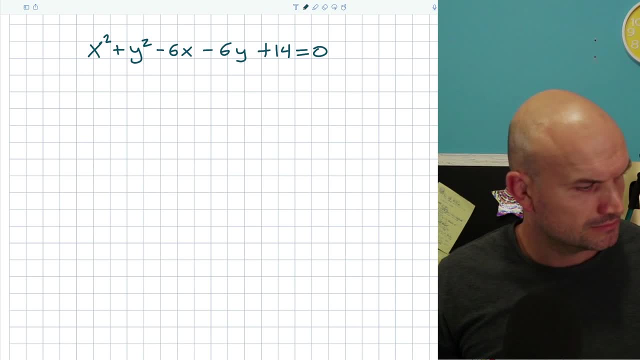 Okay. so now it's going to be the same thing: Easy, medium, hard. This is going to be finding the center and the radius of in standard form And again do the exact same thing. I just want to keep. I'm going to keep consistent with this and then we'll kind of adjust. Okay, So try to. 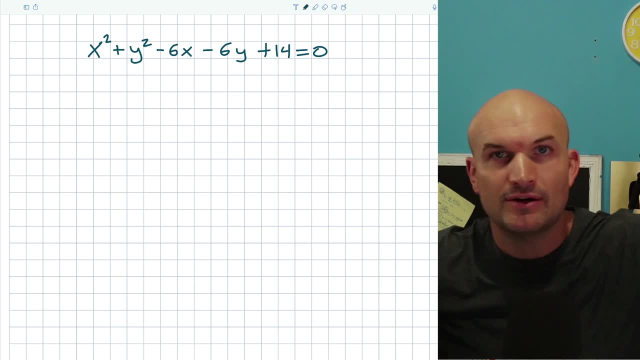 find some kind of point that's important. Three to five seconds. use text overlay right in the middle, text overlay right in the middle and then do text overlay right in the middle And then go into my standard answer room. What's up guys? All right, What's up guys In this video? what I want to do is what's up guys? 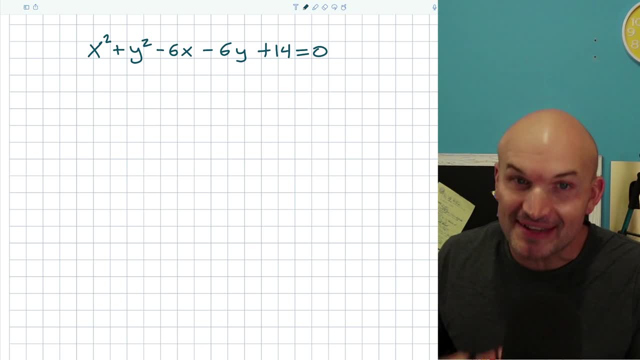 In this video. what I want to do is be able to find the center of the radius of a circle in general form, And you can see this form is not going to be very fun. What we're going to need to do in this? what we're going to need to. 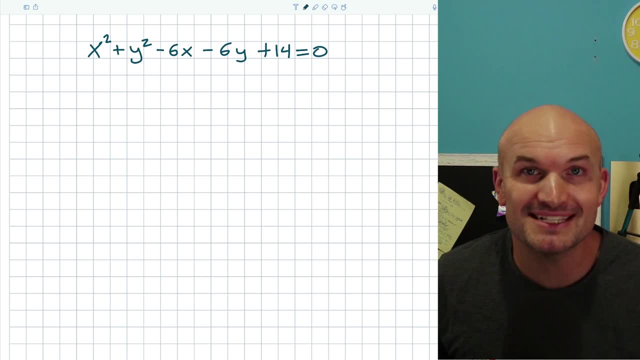 what we're going to need to do to write this from general form to standard form is to complete the square, Everybody's favorite process. So a couple of things we want to remember, like this is in this. So a couple of things we want. 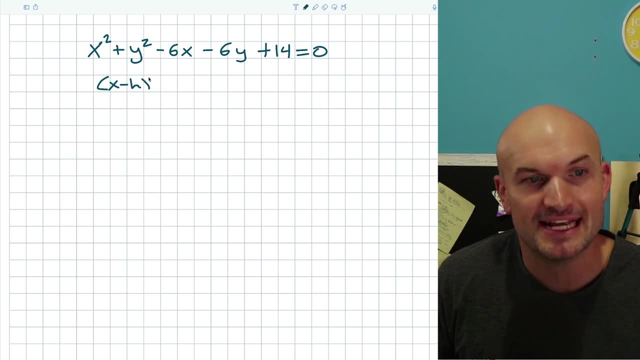 to remember. we're trying to write this into that standard form of X minus H, quantity squared plus a. Y minus K, quantity squared equals R squared right. So the center is going to be our HK. That's what we're looking for, And then we're going to look for our radius, which is not going. 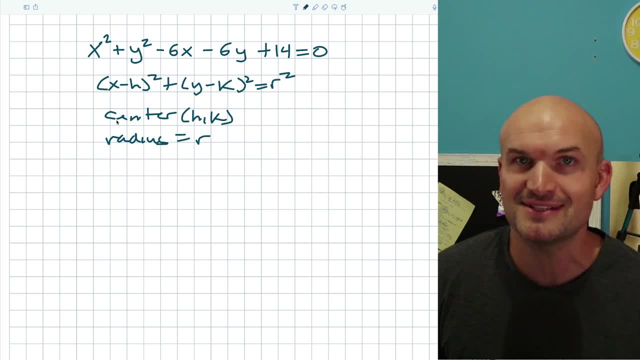 to be R squared, It's just going to equal R, So I wrote that a little bit quickly. Sorry, You can see my penmanship's kind of bad, but that's what we're trying to do, right? So what? so to get? 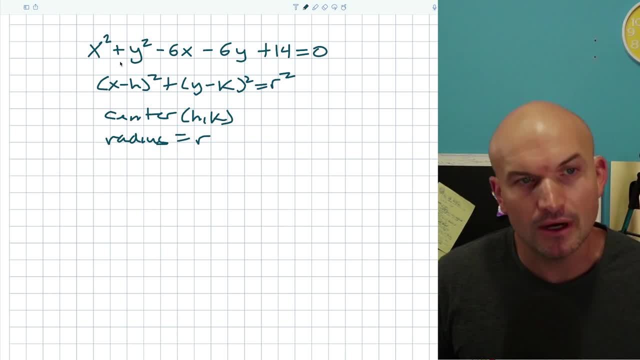 these quantities squared. that's what completing the square is going to do. All right, So the main thing I want you, first thing we're going to want to do, is just kind of group the X's and the Y's together. So therefore, I'll just rewrite the equation as X squared minus. 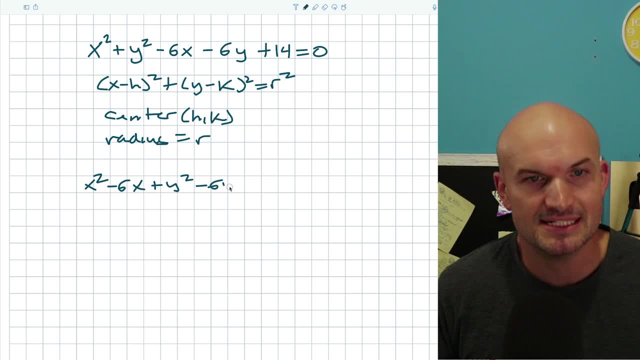 a six X and then plus a Y squared, minus a six Y. And then I'm going to get the 14 over to the other side because again we want this to be equal to the radius right. So I'm subtract the 14 to the. 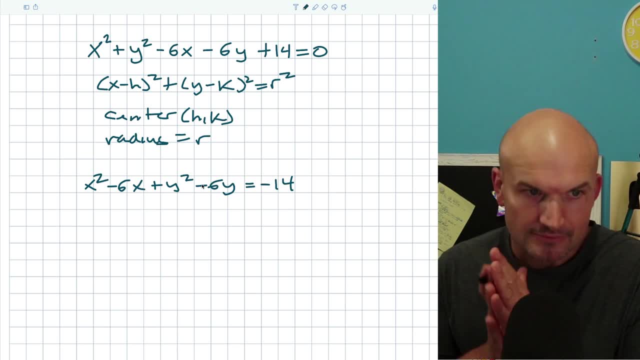 other side, That's going to now equal a negative 14.. Okay, Now it's going to be completing the square time, So what I'm going to do is I'm going to group my X's together and I'm group my Y's. 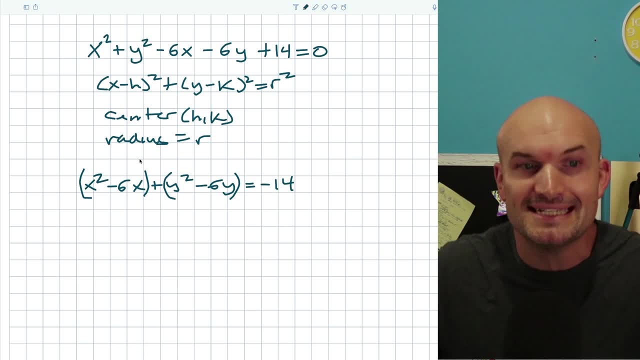 together right. So again, our goal of completing the square is creating a perfect square trinomial. Now, a perfect square trinomial is going to be a trinomial that can be factored down into a binomial squared. So to create that, what we're going to do is we're going to need to find the value C that. 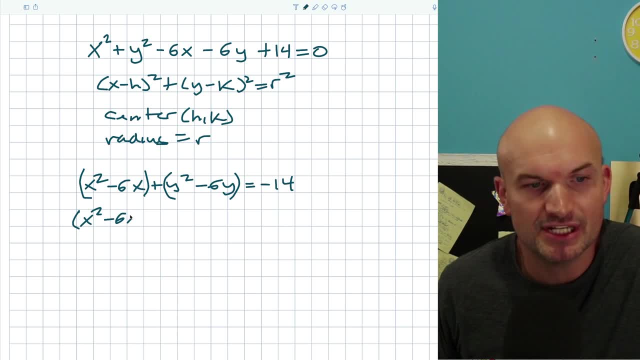 creates that perfect square trinomial. So you don't need to do this step, but I'm just going to kind of write it in, because this is kind of like the introductory example and we won't do this for the other two, but I want you to see. what we're trying to do is find this value C, that is. 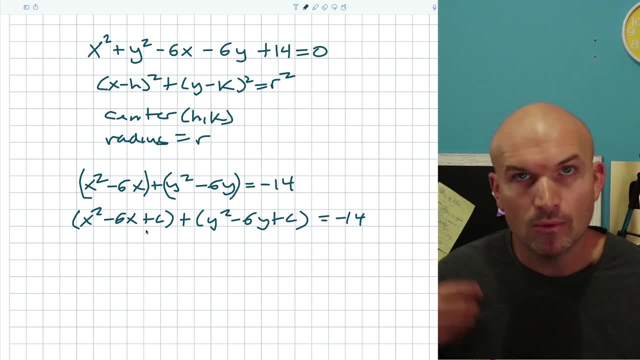 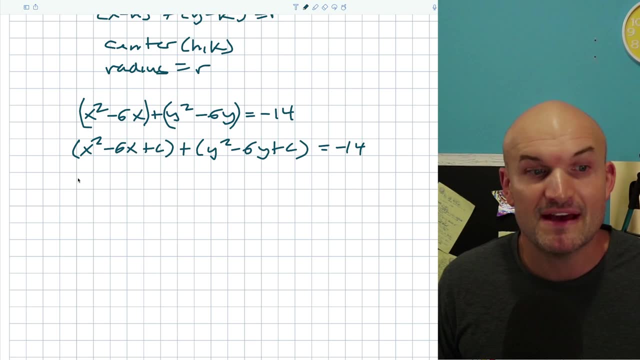 going to create a perfect square trinomial. Now, once you get good at this, you can probably do this in your head, but while you're still kind of learning or getting used to this, there is a little formula to be able to find C, and that formula is going to be a B divided by two. 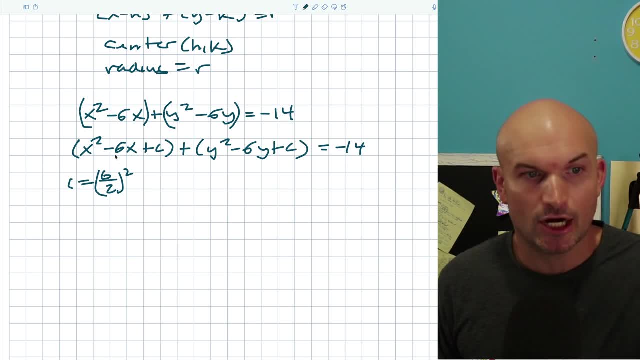 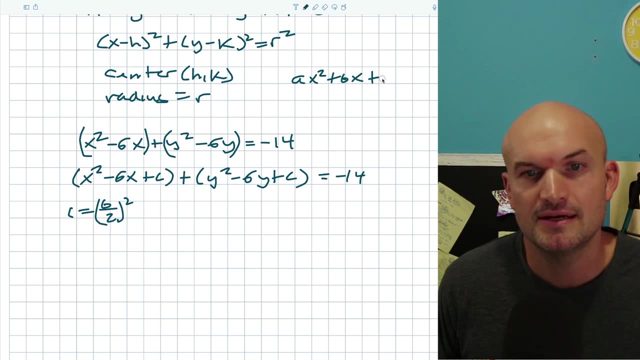 quantity squared. So all we're simply going to do in this case is going to take our B, which is our middle term, right, Remember? remember, like the standard form of a quadratic, like a X squared plus B, X plus C, right? So we're going to take our B divided by two and 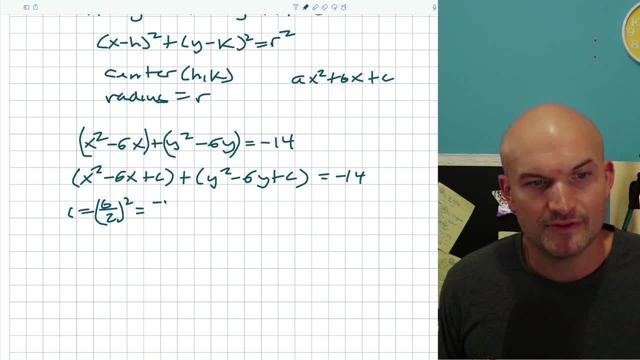 then square it. So in this case, and the first example, we have a negative three. No, I'm sorry, negative six. I was doing the math in my head. So a negative six divided by two, quantity squared. negative six divided by two is a negative three. negative three squared is going: 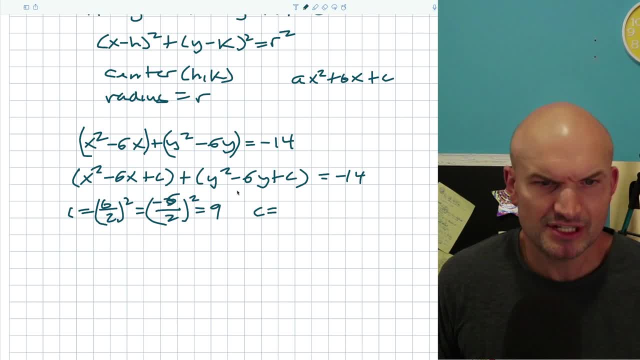 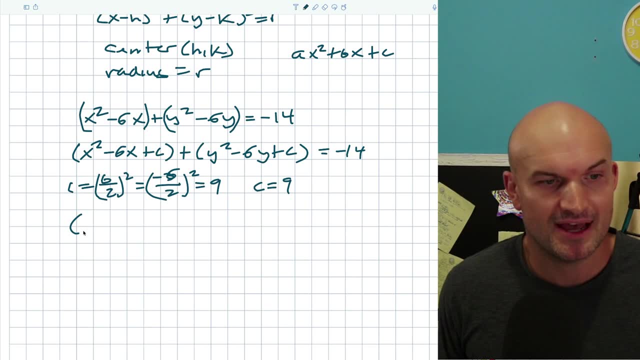 to be a positive nine. Now, in this example, we can do the exact same. Actually, you can see it's nine for both of them, right? So that's going to work for both examples. So now I'm going to replace this with a nine inside of here. So therefore I have a X squared, minus a six X. 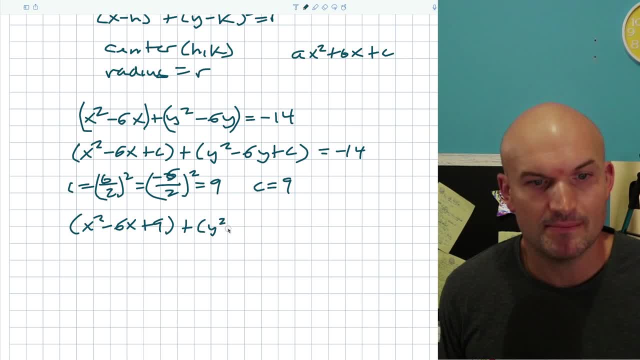 plus nine plus a Y, squared minus a six, Y plus nine equals a negative 14.. Okay, Now there's something really important I want you to recognize here. I just added a nine on the left side of the equation. Well, whatever you do on one side of the equation, 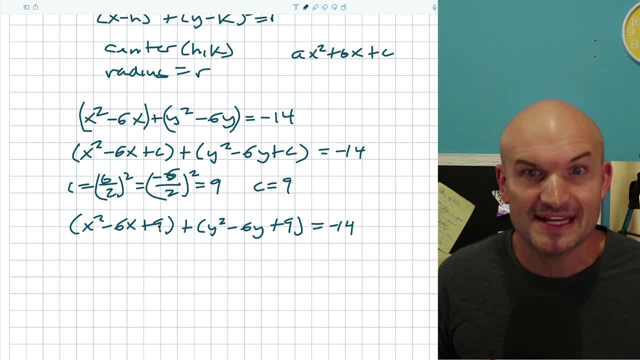 you have to do on the other side of the equation, right. So if I add a nine over here on the left hand side, then I have to add a nine over here on the right hand side, And then over here I added a nine again. So if I add a nine on the left hand side, I need to again. 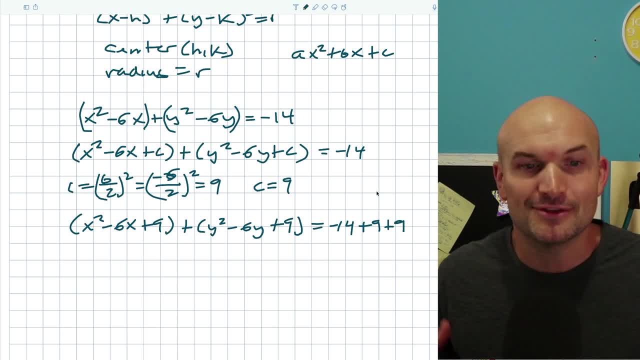 add a nine on this right hand side. Okay, So just make sure you're using those properties of equality. Now, what I'm looking at is two binomial squares, right, And the reason why these are binomial- sorry, perfect square. trinomials. And again the reason why these are perfect. 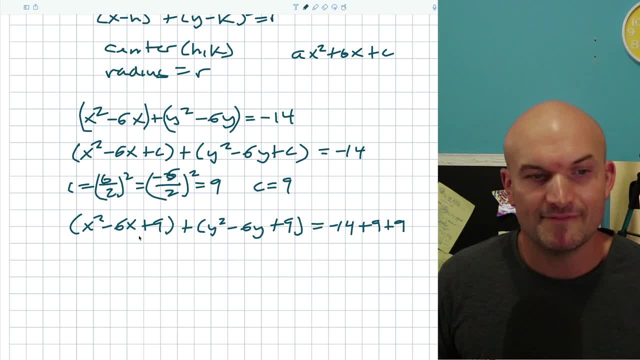 square trinomials is these can be factored down: Two binomial squared, Like if you were to look into this factor form of this, what two numbers multiplied to give you nine, add to give you a negative six and hopefully recognize that's an 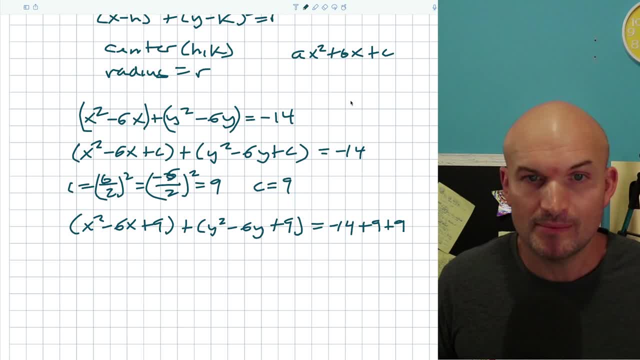 X minus three, or that's a negative three and a negative three. So the factored form of that would be an X minus three times X minus three, right? Let me actually just write this up here. So X squared minus a six, X plus nine, right? So that's going to be a X minus three times an X. 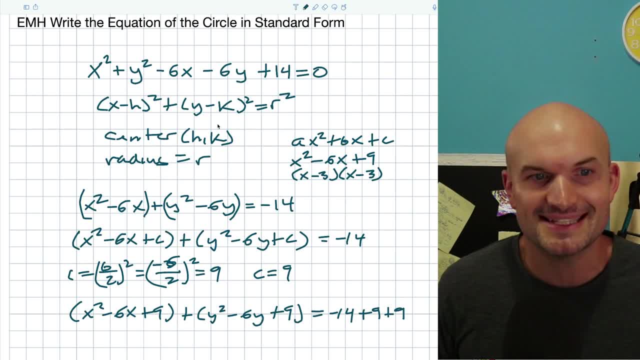 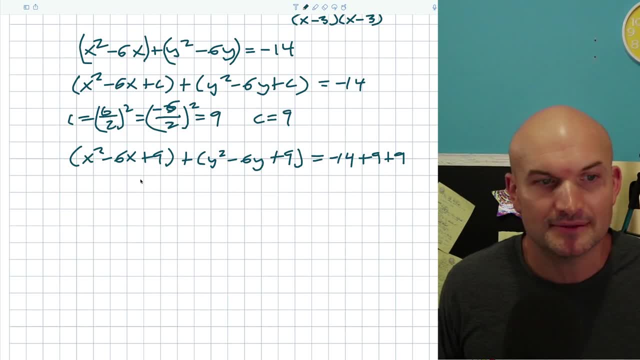 minus three. but we don't want X minus three times X minus three, right, That's not in our standard form. We want this to be a quantity squared. Well, again, it's. anything multiplied by itself is itself squared. So I can rewrite this as a X minus three, quantity squared plus a Y. 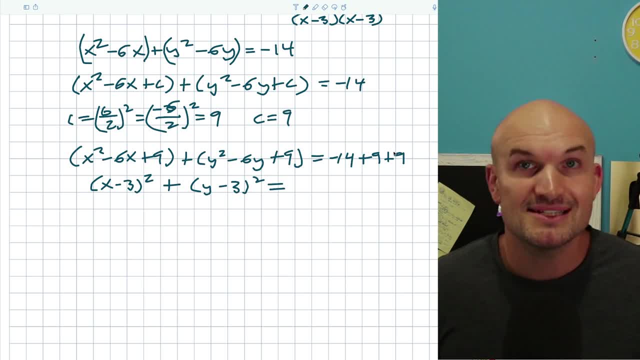 minus three, quantity squared, And that's going to equal a nine plus nine is going to be an 18 minus a 14.. That's going to be a what? that's going to be a five, five, Okay. So now what we? 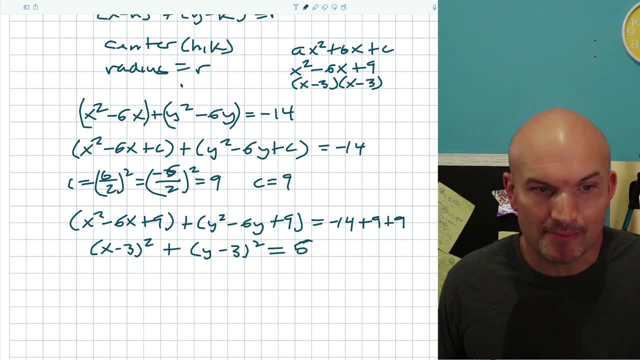 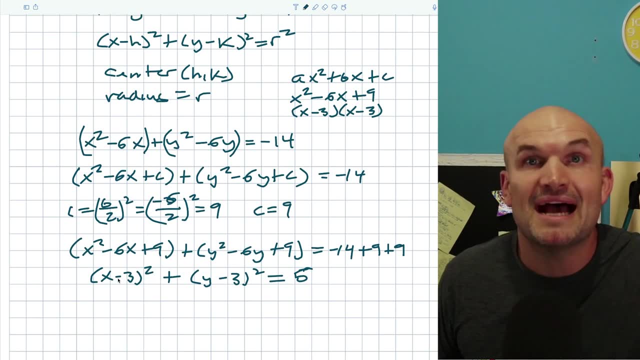 can do is just identify our center right. So again, make sure that you remember that your H and your K are actually going to be the opposite right? This is X minus H. So this is X minus H. Well, so that's X. 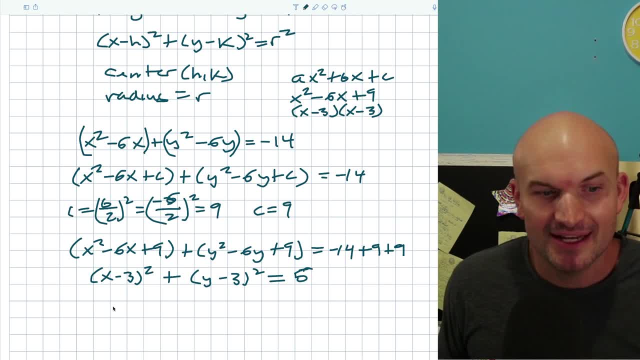 Minus H or X minus three. So what that means here is my H is actually going to be a three. Don't make it a negative three. So my center here is a positive three and my um a. I'm sorry. 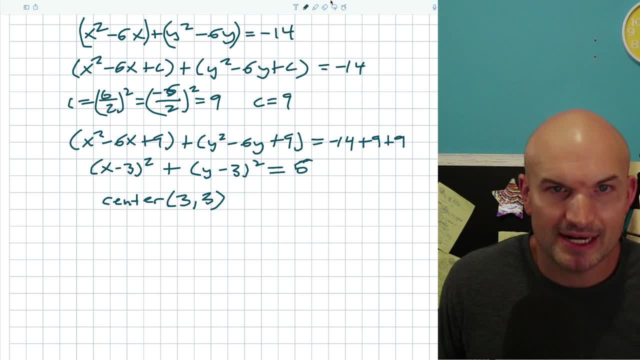 my H is a three and my K is also going to be a three. And then for the radius, I'm just going to rewrite this here for a second: make that nice and pretty. So then now my radius. here, my radius is going to be a, the square root of five, right? Because, again remember, 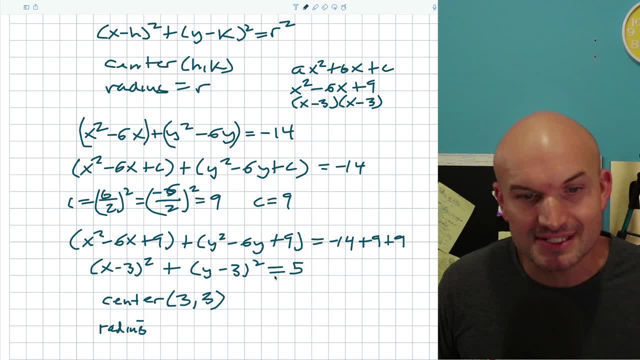 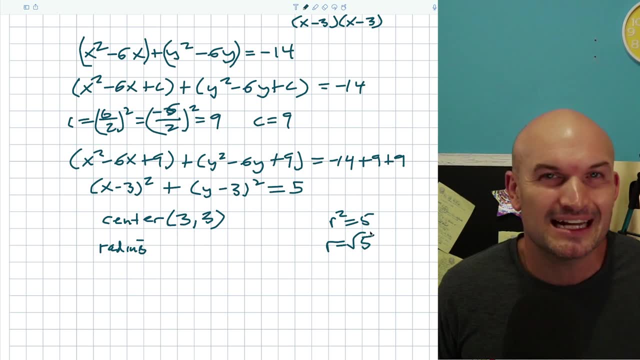 this represents R squared right. So when you have this in the standard form, that's R squared. So R squared is equal to five. So therefore, R is equal to the square root to five. It's not going to be negative because again, it's a positive distance. Um, that's the radius. 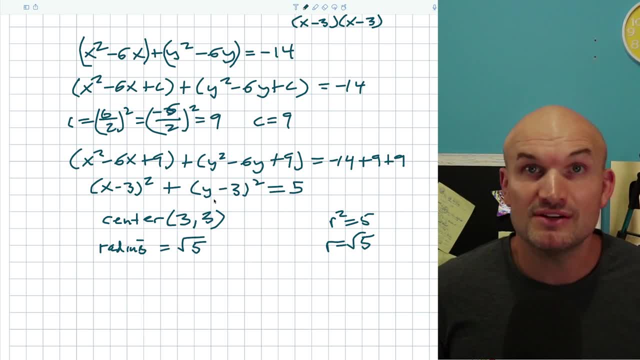 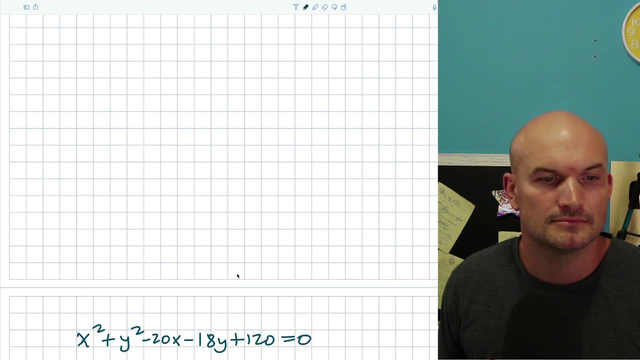 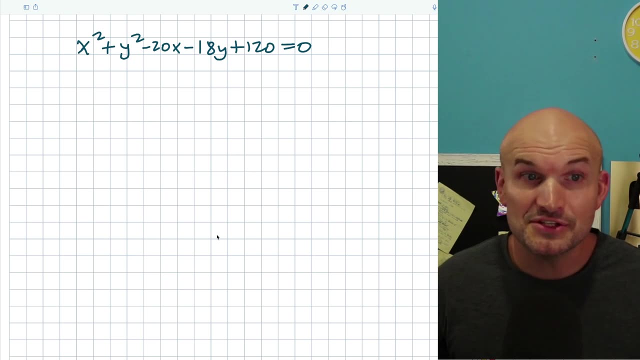 represents right. So therefore, that's going to be a positive square root of five. All right Now let's do another example. Um, again, with completing the square. I not. all right now, let's go and do another example of completing the square. You can see, we basically 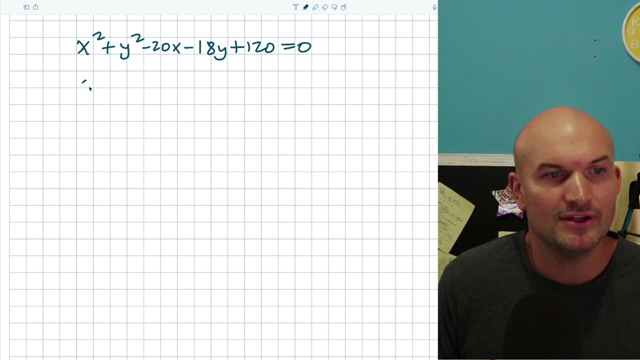 kind of have the exact same format. We're going to follow the exact same steps. The only difference here is we just kind of have a little bit of numbers, So when we're going to be completing the square, things are just going to change up a little bit. But again, the main thing I want to 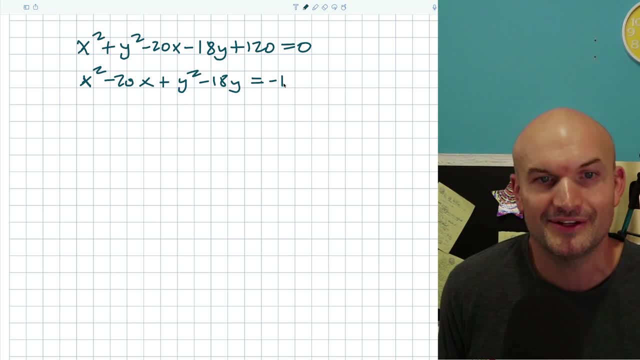 do is group my terms and get my 120 here over to the other side. All right, Then I'm going to use my parentheses to kind of group them. You don't really need to use a parentheses, but again, I just like to kind of have things grouped in there. So I'm going to do that. So I'm going to do. 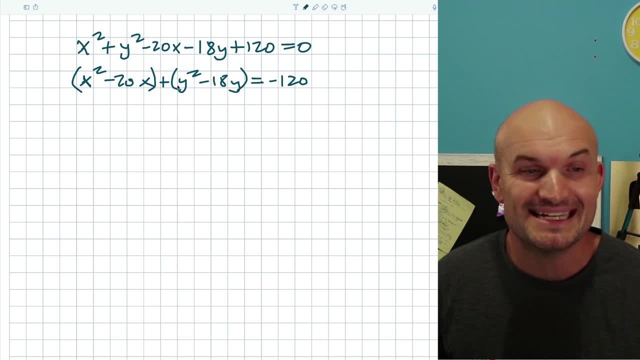 this format. So now I need to complete the square. Now, notice, my B is different in these two equations. So therefore, I'm going to, um, I'm going to find, or, I'm sorry, not my B. Yeah, my B is different. So therefore my C is going to be different, right? So my C in this left-hand. 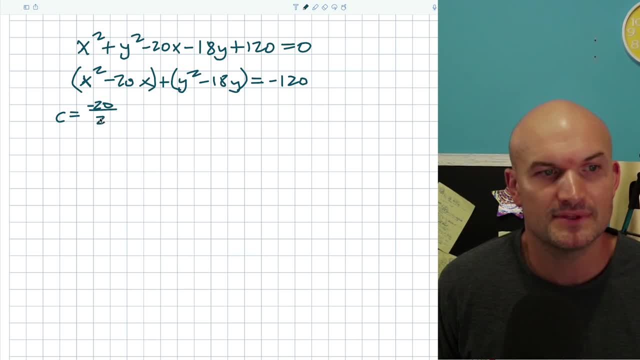 one is going to be a left-hand bracket is going to be negative. 20 divided by two, right Quantity squared. So negative 20 divided by two is going to be a negative 10, negative 10 squared is equal to a hundred right. So that's where I'm going to add inside of that parentheses, And then over here: 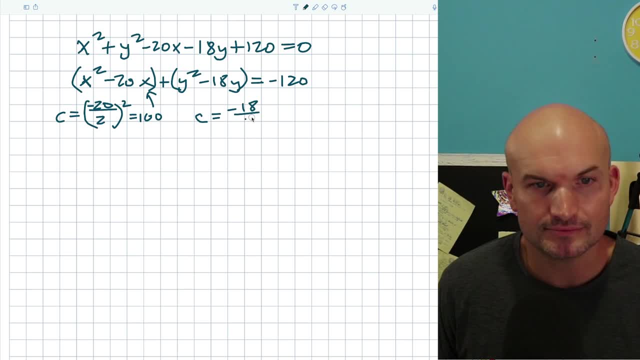 I'm going to have a. C is equal to A negative 18 divided by two, And then again that's going to be quantity squared. You can see how the negative doesn't really make sense. It doesn't really matter because you're going to. 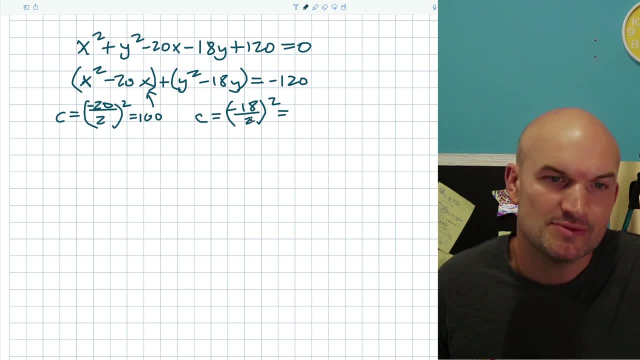 be squaring things anyways. Um so, negative 18 divided by two is going to be a negative nine. Negative nine is going to be squared. It's going to be a positive 81.. Okay, And that is what we're going to add inside there. But remember, whatever we add on the left-hand side, right, Don't forget. 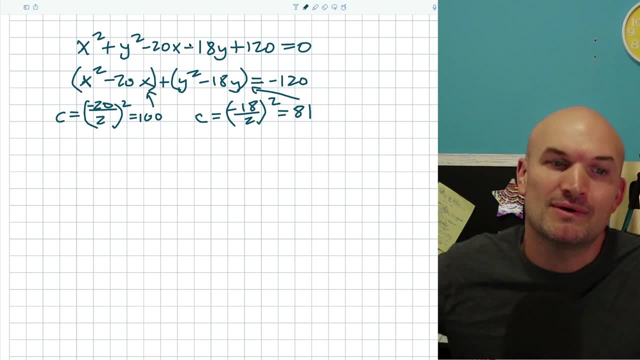 please don't forget: whatever you do on the left-hand side, you have to do on the right-hand side. Okay, So, um, now I can write this as a a X squared minus a 20X, plus um, plus a hundred, And then over here I'm going to have a Y squared. 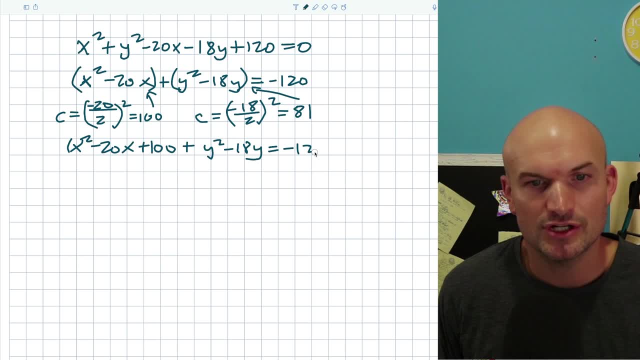 minus a 18Y is equal to a negative 120 plus a hundred plus an 81, right, Be very, very careful. Make sure you don't forget to do that. All right? Um, I added a little parentheses here, but we don't really need that little parentheses in this case. Like we can. 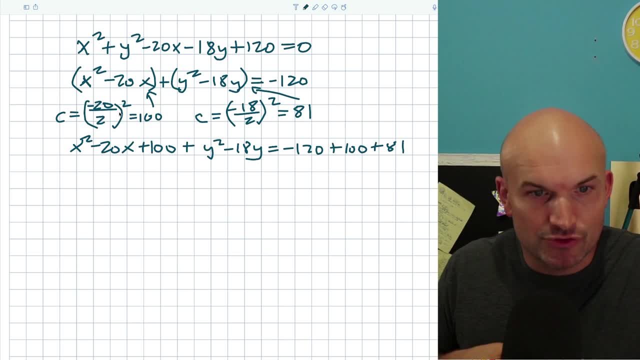 hopefully you can recognize these factories. So hopefully you can recognize that you created. I don't know I forgot to write this in there, right, Plus 81. So I forgot to write that in there. So let's move this over just a little bit more and let's write plus 81. So be very careful to write that in. 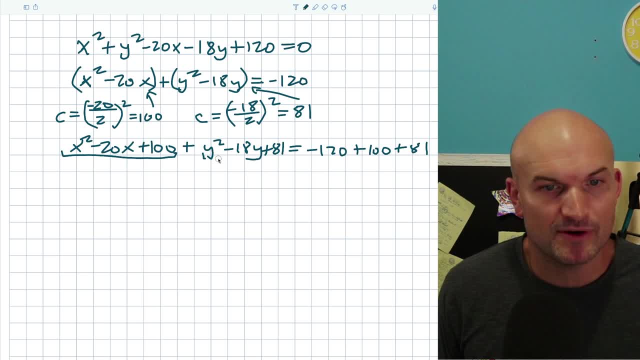 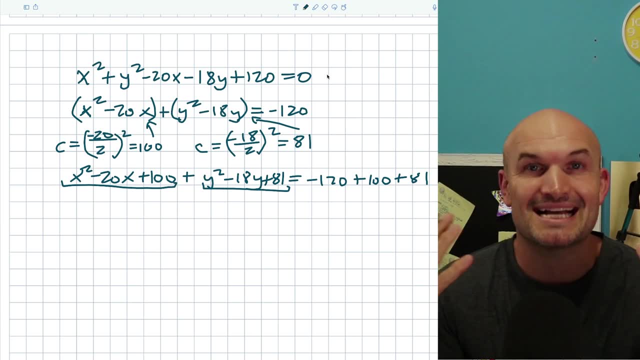 Okay, So remember, this is a perfect square trinomial and this is a perfect square trinomial. Remember, all perfect square trinomials can be rewritten as binomial squared. So, basically, what you're thinking of is what is the exact same number that multiplies. to give me my last term, 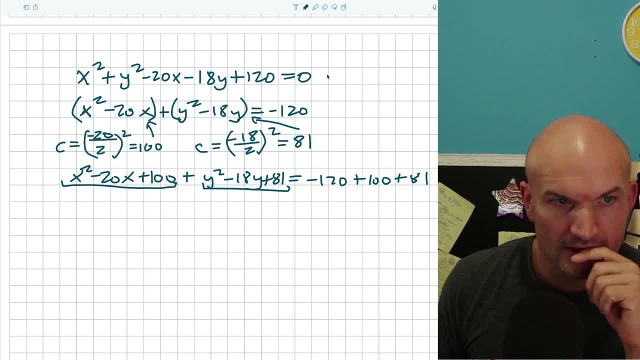 but then adds to give me my middle. So in this example you're thinking: all right, what two numbers that are exactly the same ad to give me a hundred. that multiplied to give me 20.. Hopefully you recognize that's going to be our. 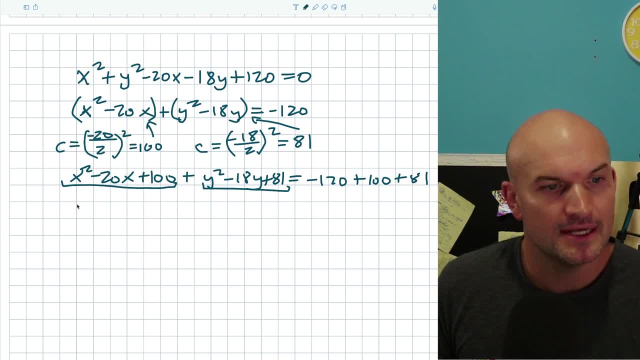 negative 20.. Hopefully you recognize that's going to be a negative 10 and a negative 10.. So in this case I can rewrite this as a X minus 10, quantity squared. Well, what about 81?? What two? what numbers multiplied? exactly the same, that multiplies to give you 81 and that adds to. 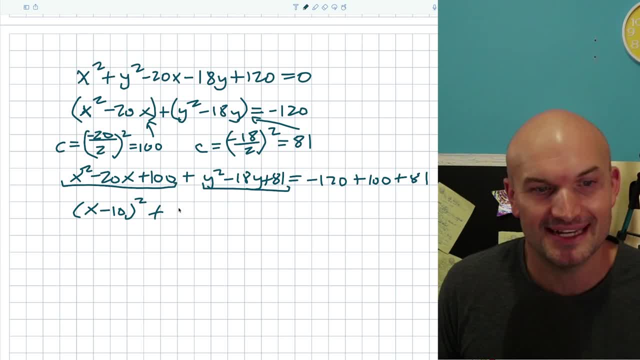 give you an 18.. Hopefully you recognize. you're like: oh all right, this is going to be a negative. uh, negative nine, So X minus nine, quantity squared, And then over here we can just going to combine these. So negative 120 plus 100 is a negative 20.. Negative 20 plus 81 is going to. 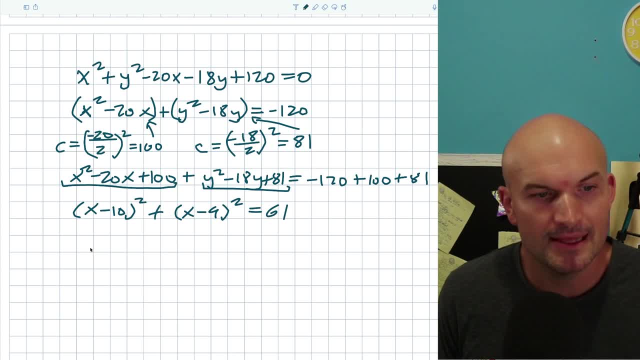 be negative. 20 plus 81 is going to be a positive 61. So in this case my center again is going to be the opposite right. So it's X minus H, X minus K. So therefore my H is going to be a 10. My K is: 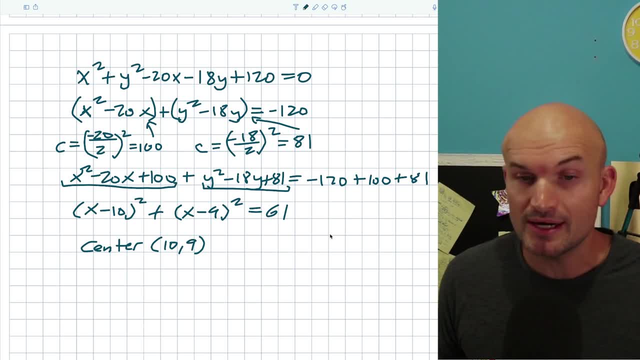 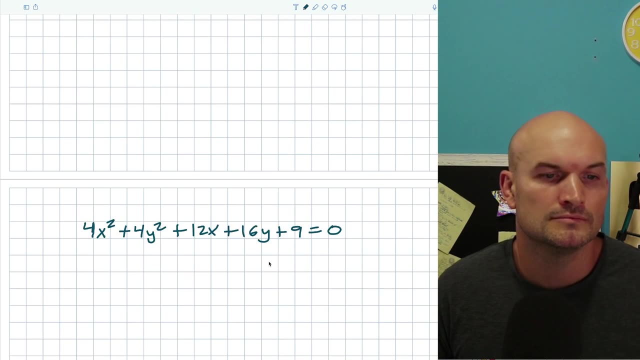 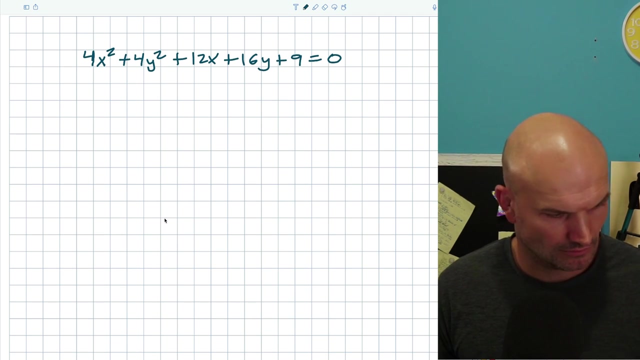 going to be a nine, and then 61 is equal to an R squared right. 61 equals R squared per the formula, So R equals a square root of 61.. So, therefore, my radius is going to equal a square root of 61.. All right, Now it's time to have some real good fun. Now it's time to have some. 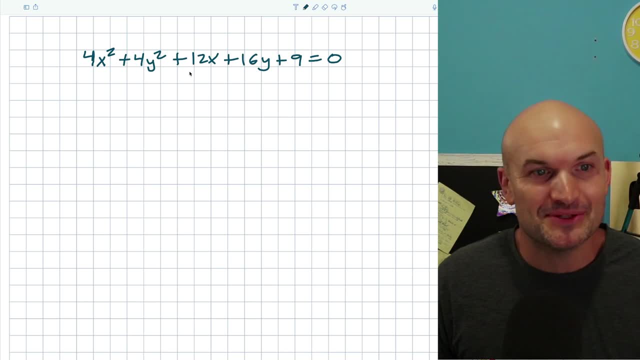 real good fun With completing this square. So in this example you can see we have a lot. So in this example you can see we have a very similar situation. However, in front of the X squared and the Y squared, we do have this four. So let's go ahead and see when we're going to address this, But for 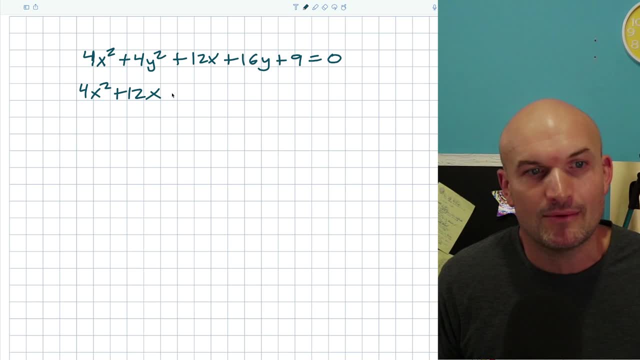 right now, let's just go ahead and group everything together, right? That's the main thing I want you to kind of focus on First of all is getting the X's and the Y's together and getting that nine over there on the other side. Okay, Now, what I want to do is I need to complete the square and 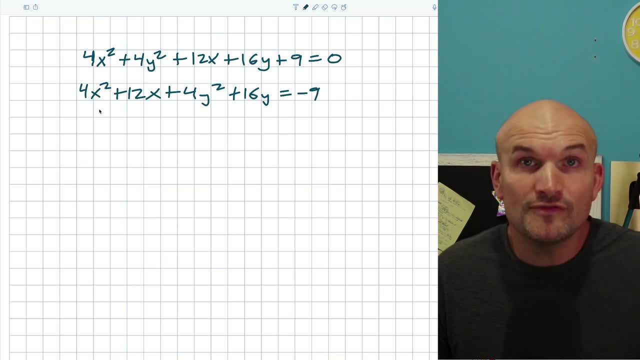 hopefully and hopefully you remember to complete the square. when you have a coefficient, you have to be able to factor that number out right. And now you could divide everything by four here on the left-hand side and then on the right-hand side. But again, sometimes it gets a little confusing when you 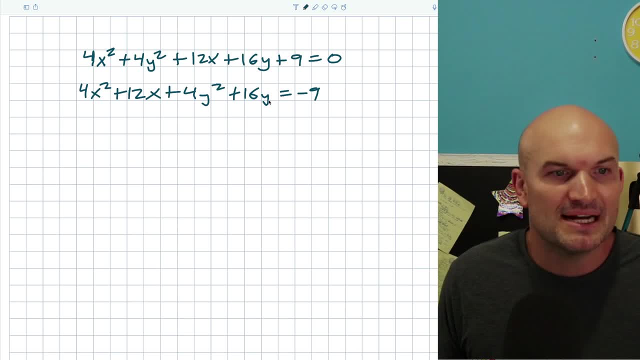 are creating a fraction on the right-hand side, but you can definitely do it Actually, yeah, let's just go ahead. Okay, Yeah, Now, hopefully you remember when you are completing the square, when you have a number in front of your quadratic term, you have to get rid of that number. So there's a couple of different. 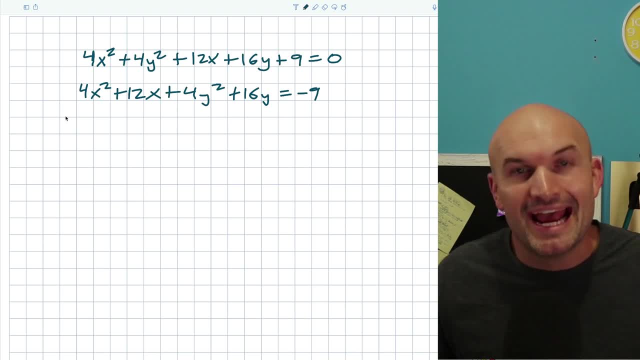 ways you could do that. You could factor out that number or you could divide everything by that number. And now, in this case, what I'm going to simply do is I'm actually going to factor out that number. Whenever I am solving, I usually like to divide out that number, But in this case, 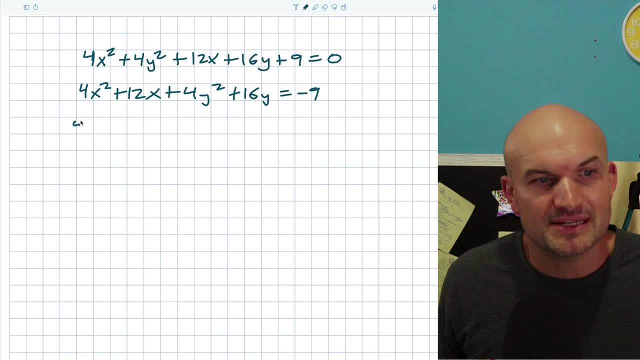 I always prefer to kind of like factor that out, right. So what I'm going to do is I'm going to factor out the four, And when I do that I get an X squared plus a X squared. So I'm going to do that. 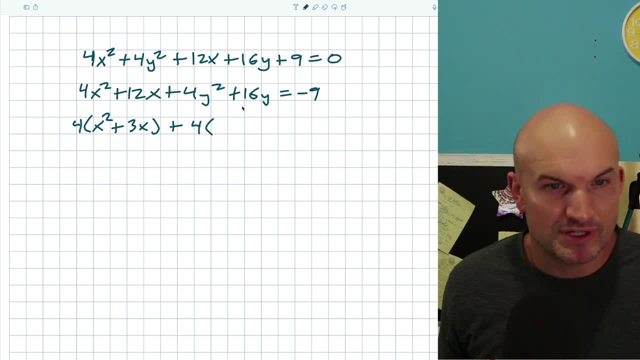 three X, And then over here, when I factor out that four, I'm going to be left with a Y squared, plus a four Y, Okay, And then that's going to equal a negative nine. Now you can see, I kind of have those parentheses which I was looking for, right, Remember we? 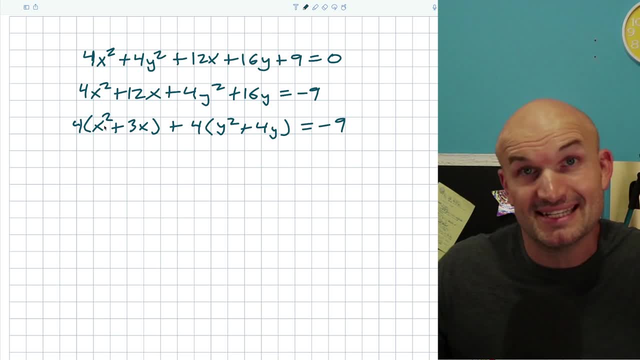 in the first example, I wrote parentheses around those terms. And then we are at first. in the second example, we wrote parentheses around those terms And then we said: all right, what is our? let's go ahead and find our C. So again we're. we're taking our B, dividing it by two, and 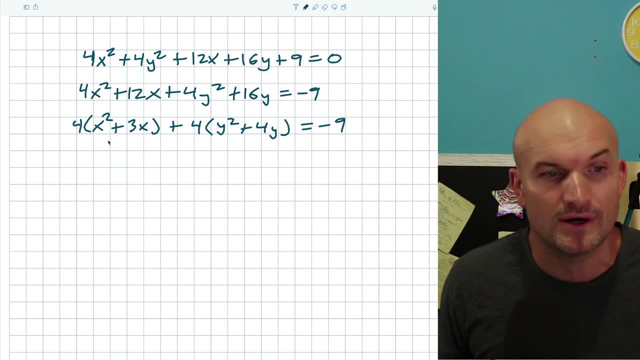 squaring it right. This four is going to come back, So do not forget about the four. Um, let's go and find our value C. that's going to um, create the perfect square trinomial. So in this first um kind of parentheses, I'm going to have a three divided by two. 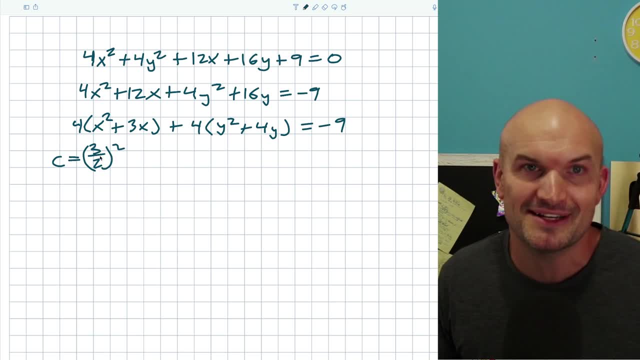 squared. Now the problem here is: two does not evenly divide into three. right, You can't actually divide that out, but that's okay, You're just going to have a fraction. So a three divided by two, quantity squared, is going to be a nine force. Okay, So that's what's going to be added. 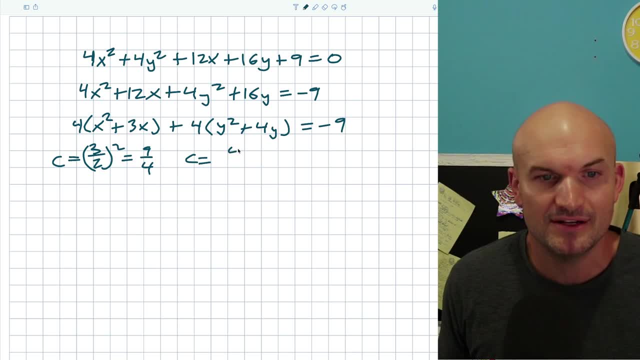 inside that parentheses, And then over here. this one is thankfully not too bad: Four divided by two: quantity squared. right, We're taking this: four divided by two squared, So four divided by two is two. two squared is four, So that equals four. Okay, Now remember: whatever we do, 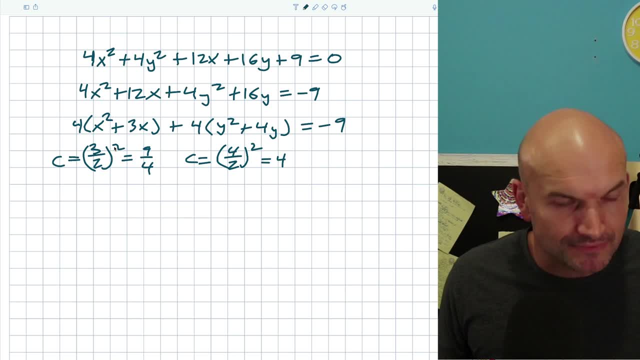 on the left-hand side. we have to do on the right-hand side, right, Don't forget about that. Okay, So, um, let's go ahead and write these numbers in over here. So I'm going to do a four times a X squared, plus a three X plus a nine force, And then over here I'm going to have a. 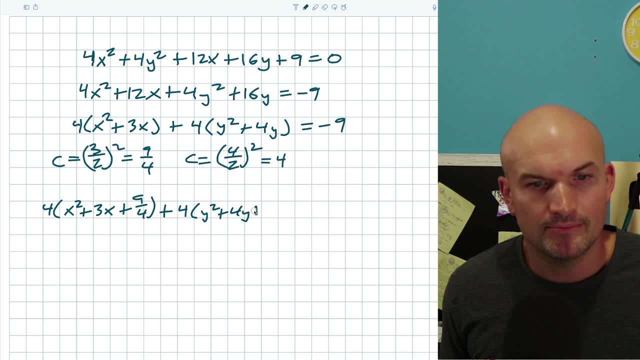 four times a Y squared plus a four Y plus four. Okay, And then over here I'm going to have a negative nine um plus a nine force. Now here's where I got to start, So I'm going to have a. 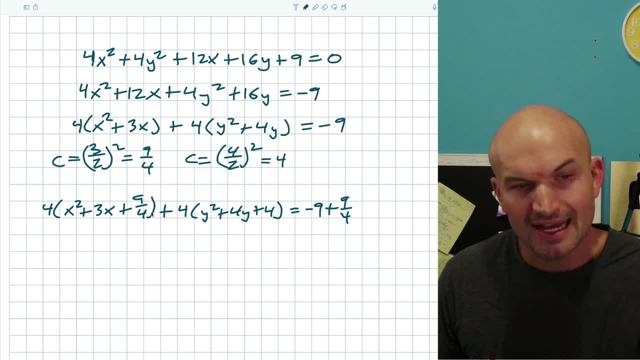 stop, because actually something very, very important just happened. I didn't actually add a nine force on the left, on the left-hand side, I added a nine force That's actually being multiplied by four right, If you remember, in the previous examples I just added something. 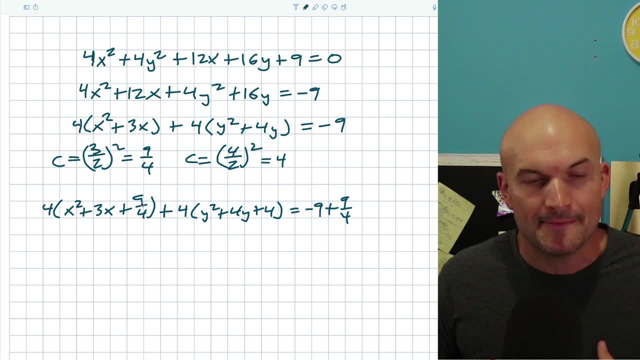 inside of a parentheses, and that was it. There was nothing that the parentheses was being multiplied by. In this example, though you can see, this nine force is actually being multiplied by the four, So therefore, remember: whatever you do on the left-hand side, you have to do on the right-hand. 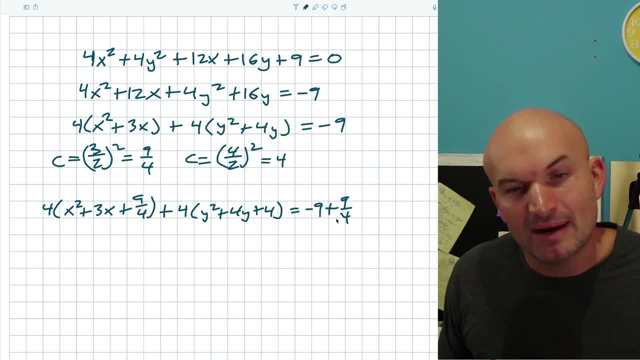 side. So if my left-hand side my nine force would be multiplied by four, Then when I add a nine force on the right-hand side, I also need to multiply that by a four, And then I'm going to follow that exact same scenario over here with this example. So I'm adding a four right, But 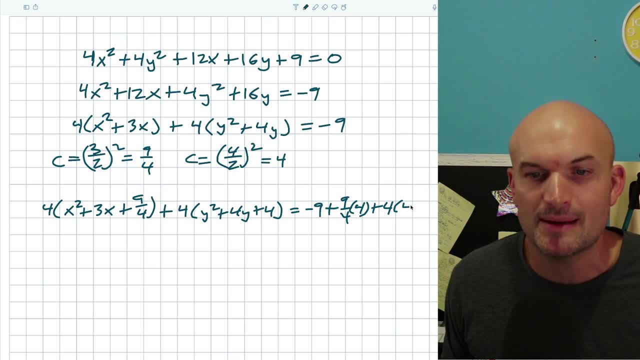 again on the left-hand side, that four is being multiplied by four, So I'm going to need to multiply by four once again. Okay, So now let's go ahead and factor this down. Now this looks very difficult to factors, So I'm going to give you a little bit of trick, but I'm going to deal with. 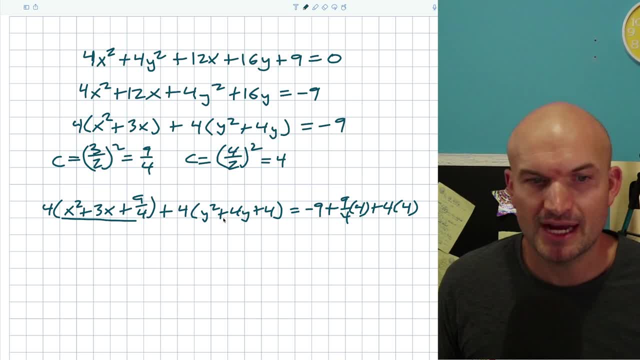 that in just a second. So this one, hopefully, is a little bit easier, right, You recognize this to be what number multiplied to give you what same numbers. the exact same multiplies to give you four. that adds to give you a four. right, That's going to be a two. 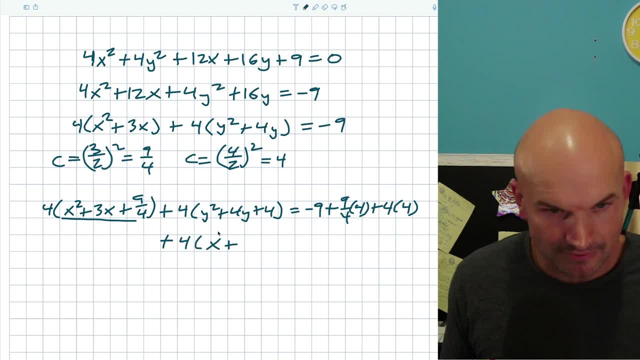 So hopefully you recognize you're like all right, that one's kind of easy X plus. let's just see X plus. what am I looking at? X plus X plus two quantity squared. Okay, Now there is something kind of interesting though that I actually didn't do. I forgot to do this. 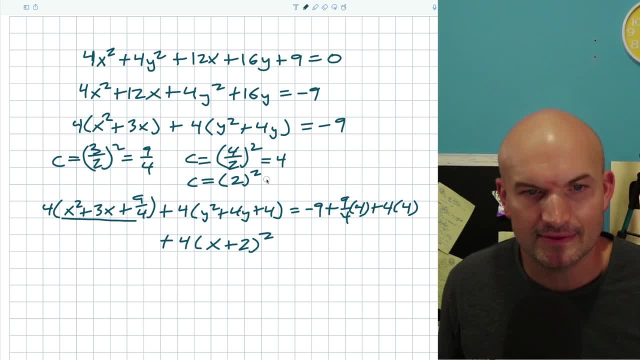 two quantity squared. Okay, There's actually something that I want you to kind of take, a relationship that I didn't talk about up to this point, because a lot of times you should be able to factor these. But in reality, what's happening is when you go from a perfect square trinomial- 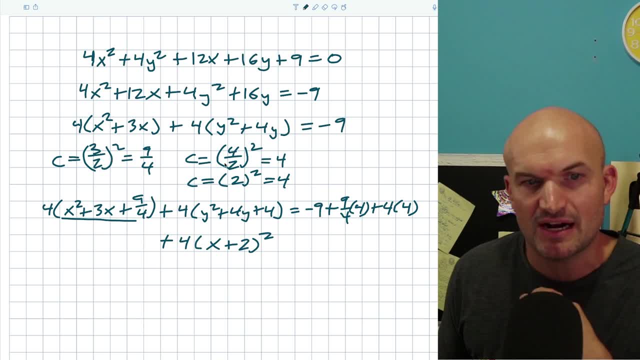 down to this binomial squared. what I want you to recognize is this: B divided by two gives you the exact same term inside of your binomial squared. So if you want to know what this factor form is, a lot of students would kind of give up and be like I have no idea how to. 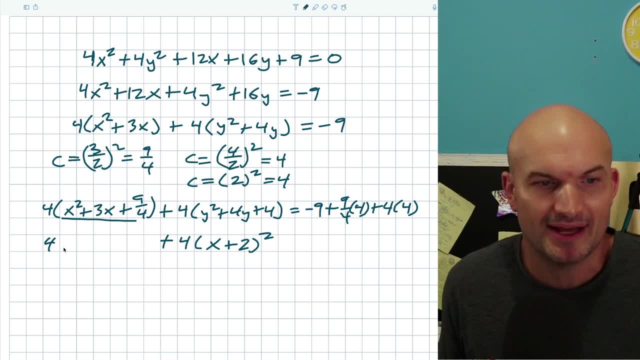 factor that, Which, again, yeah, I totally get it Like how would you be able to go ahead and factor this? However, if you can recognize that my, whenever I take a B divided by two, whatever that value is, that is going to be what's in my binomial. So I'm going to take a B divided by two. 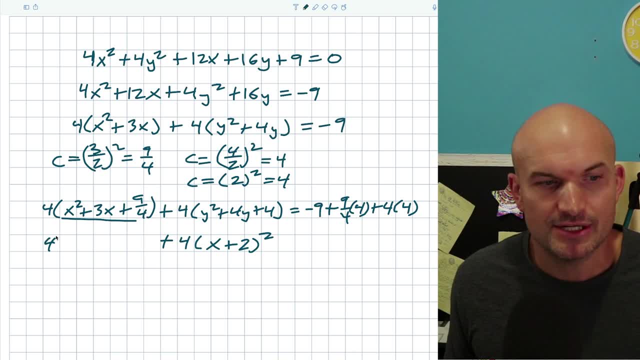 my binomial. So three divided by two is just three divided by two, right? So guess what? This is X plus a three halves. Now you might say it was that easy, Like are you sure? Well, let's go. and. 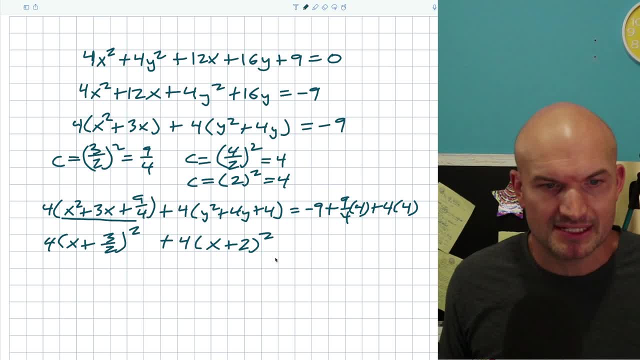 check it Three halves times three halves. right, If you were to expand this out? right, Because again, X plus two squared is X plus two times X plus two. So if you were to expand this out, watch this X three halves. Um, let's actually go ahead and do this, um on the side. So yeah, 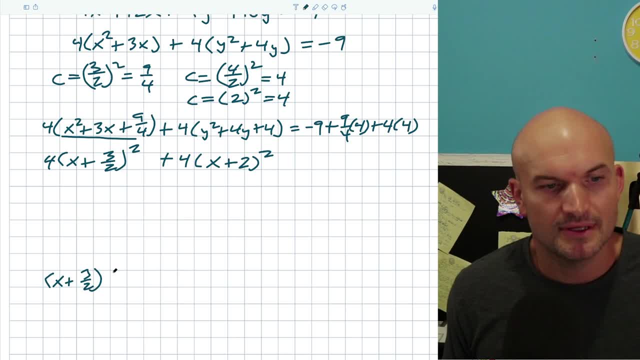 let's just do it down here. So if I did X plus a three halves times a X plus a three halves, all right, X times X is X squared right. We know that. Now what happens if I did a three halves times three halves, Well, that's going to be a nine fourths. Isn't that what you were looking? 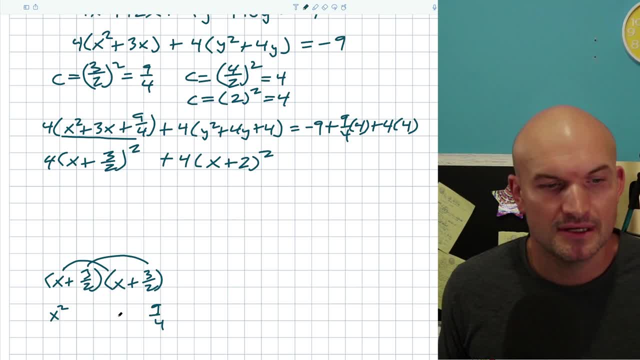 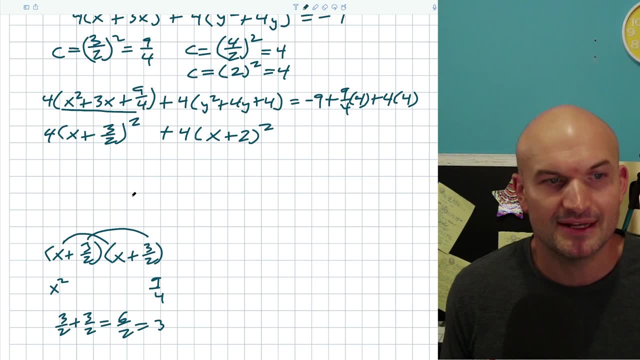 for Yeah. And then what happens if I took a three halves plus a three halves, right? So three halves plus three halves. So three halves plus three halves is equal to a six halves, which is equal to a three. Is that the middle term? Yeah, it is. So. that's all you got to do is take your B divided. 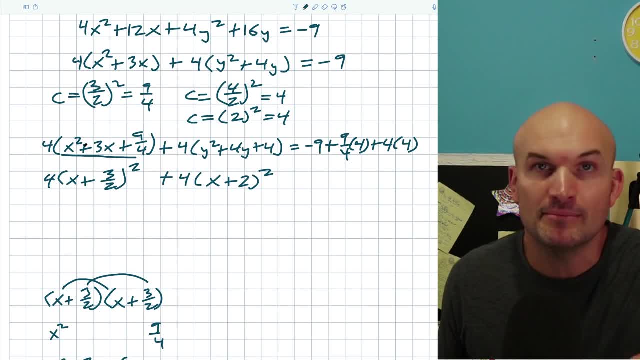 by two. And again the middle term of your binomial has to match the middle term of your trinomial. All right, So that is an easy way to kind of get by it Now over here. um, let's go and see what I have. So I have a nine fourths times nine times four. So 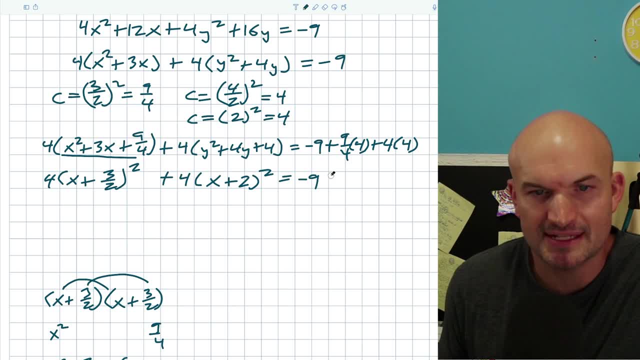 those are going to divide out. So I have a negative nine, Um, and then that's going to be plus nine, And then four times four is going to be a 16.. Okay, So negative nine times positive nine is going to be zero, So that's just going to equal a 16, but we're not done yet. So let's go and 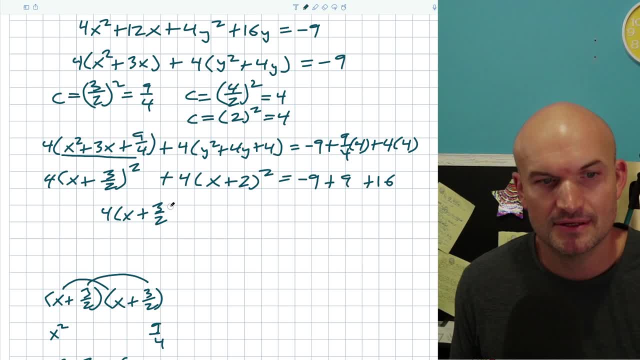 condense this Now again, remember we have these fours plus a three halves quiet squared, plus a four times an X plus two quiet square for F equals 16.. Remember the equation circle is: X minus H, quantity squared plus Y minus K quantity squared equals R squared. 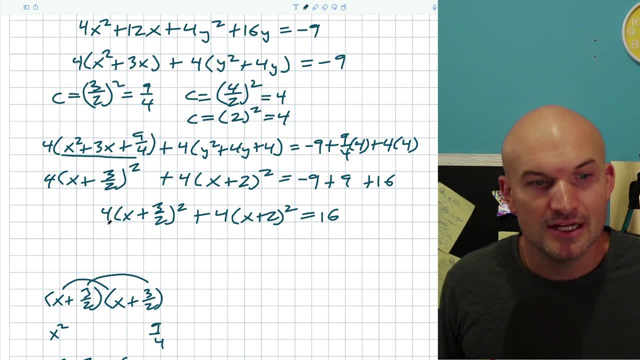 Did not talk about anything in front of the, in front of the X or the Y. So we have to divide everything on the left-hand side by four and over here by four. Now again, we're not going to divide inside the parentheses, because these are being multiplied by four. So what's going to happen? 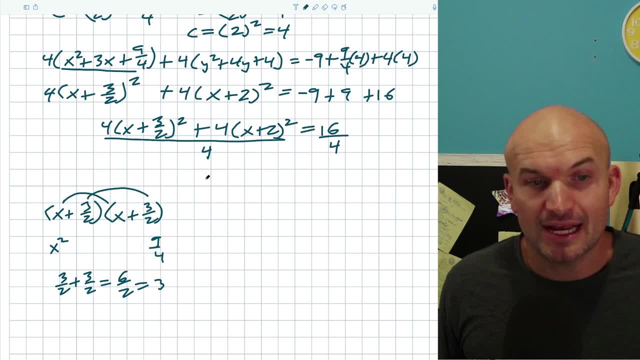 though, is those fours are going to get divided out. The other thing I want you to recognize is remember the form is X minus H. We don't have it in minus, We have it as a plus, right. So again, just remember we can always rewrite. Remember we can always rewrite like X plus a three halves. 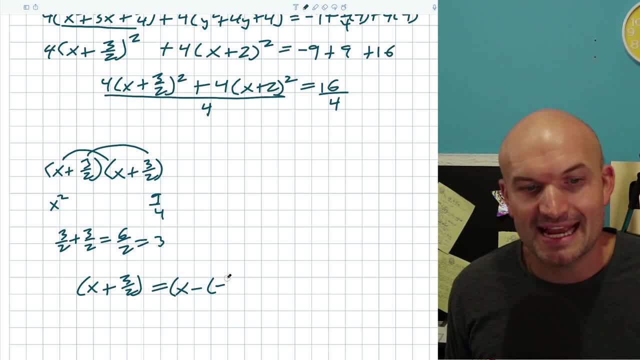 That is the same thing as an X minus a negative three halves, right? So it's very important to recognize that my H and my K in this example are actually going to be a negative three halves and a negative two. So when I do divide by my four, though I can rewrite this as an X minus, I'll. 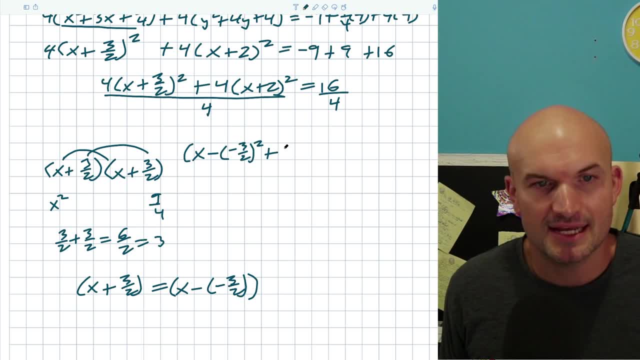 just rewrite it like this So you guys can kind of see: So that's going to be plus a, let's say X, minus a negative, two quiet squared And that's equal to four. Hopefully you recognize like minus a negative is still a positive right. So hopefully you see now. 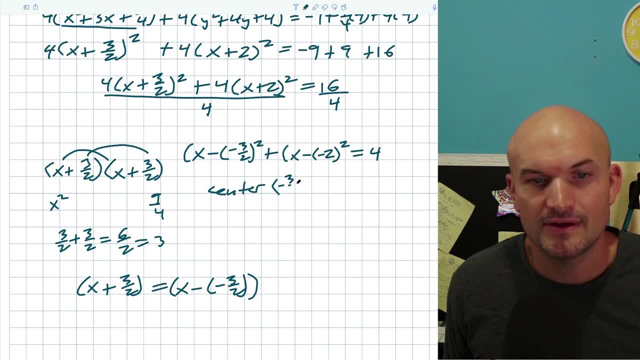 that the center in this example is going to be a negative three halves and a negative two, And therefore I'm going to have a radius is equal to a two. So if finding the center and the radius was helpful for you in this video, then you're absolutely going to love actually writing the. 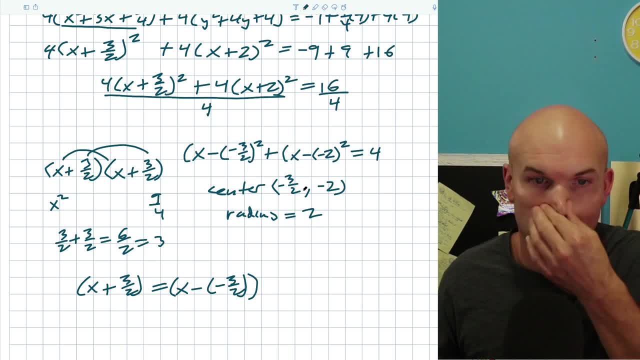 equation of the line which I'm going to get into the next video. No, you're actually, you're actually going to love, you're, you're going to love writing the equation of a circle which I'm going to get into in the next video. Now, let's not get into the next video, So this will help.